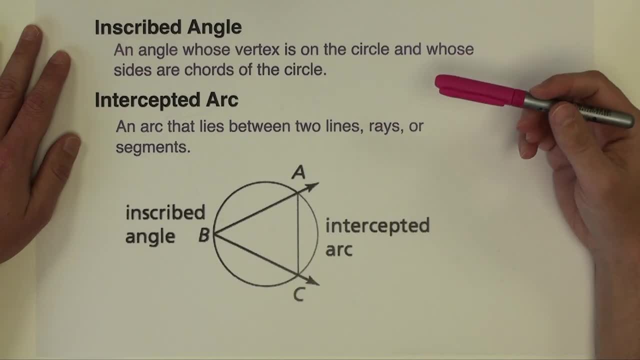 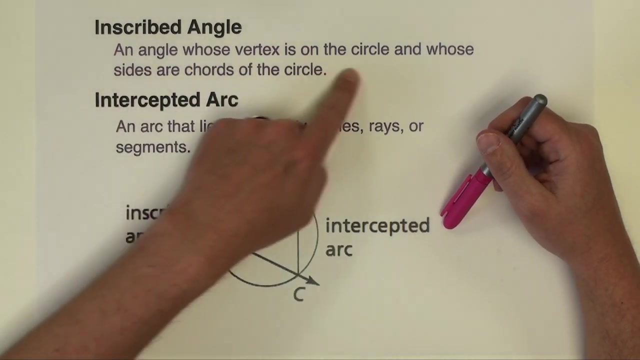 vocabulary of what these things actually are. Okay, first up is the inscribed angle. So different from a central angle is going to be the location of the vertex of this angle. With the inscribed angle, the vertex of the angle is on the circle, whereas before, with the central angle, was at the center. 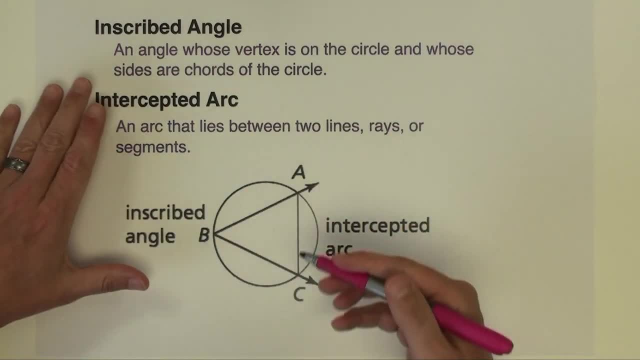 So we're just moving where the vertex is located. So you see this angle here, this angle ABC, and looking at this diagram, you can see that the vertex of the angle, point B, is actually on the circle instead of being in the center of the circle, like we saw. 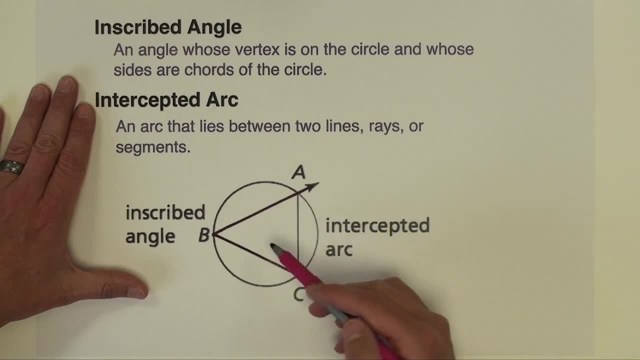 In the previous couple of videos now notice that when I draw that the sides of this angle have hit the circle at two places and if we look between those intersection points we have what we call an intercepted arc. So we're going to begin this video tutorial on a theorem that will tell us 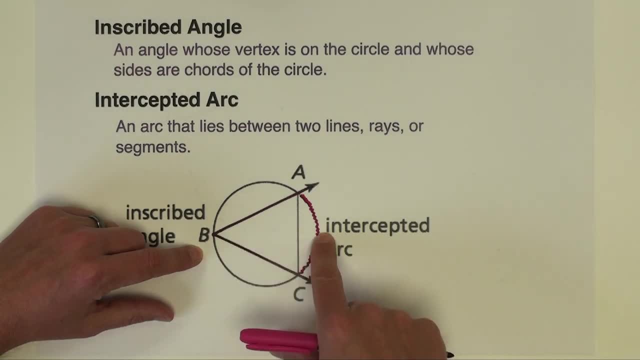 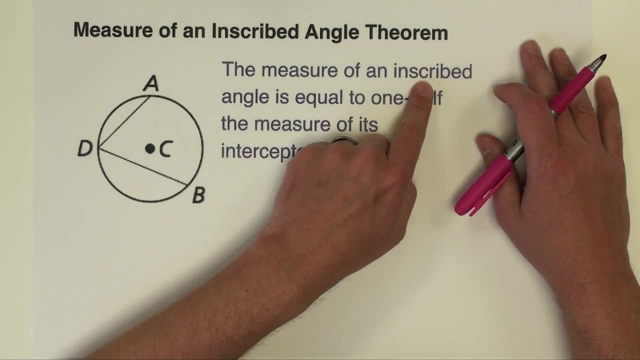 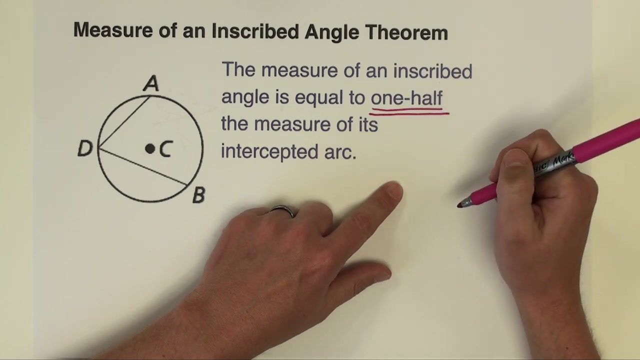 the relationship between the measure of this angle and this intercepted arc. All right, here is that theorem to describe that relationship for us. This theorem says that the measure of an inscribed angle is equal to one half the measure of its intercepted arc. When I 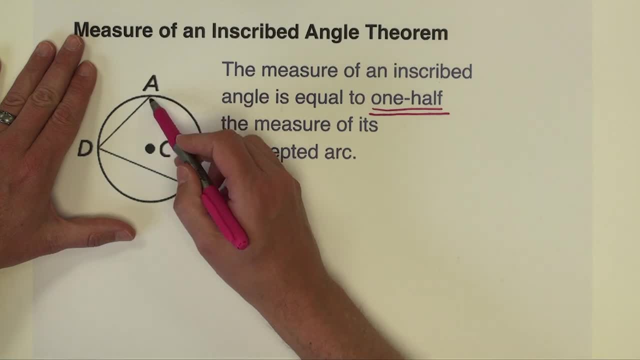 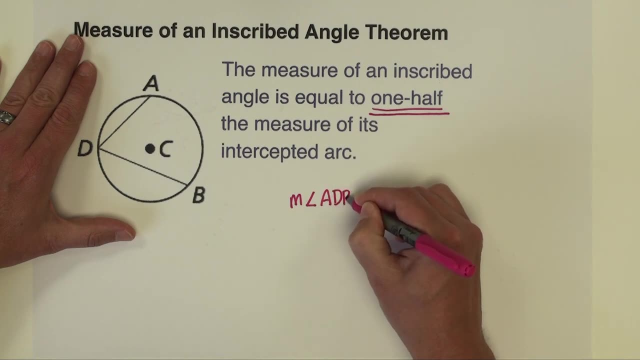 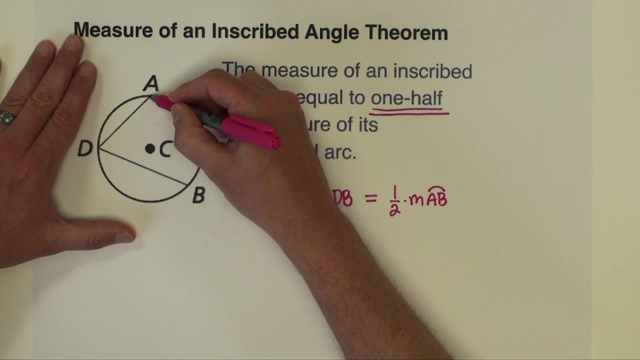 look at this particular diagram: the measure of the inscribed angle, so let's do this- the measure of angle ADB. okay, So this angle here is equal to one half. the measure of angle ADB, measure of the intercepted arc, which is AB. In other words, if you think of it like this, 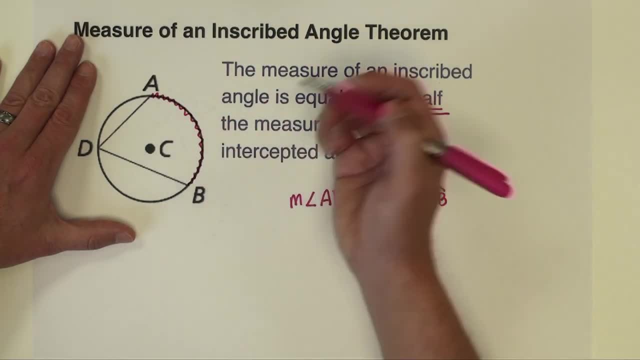 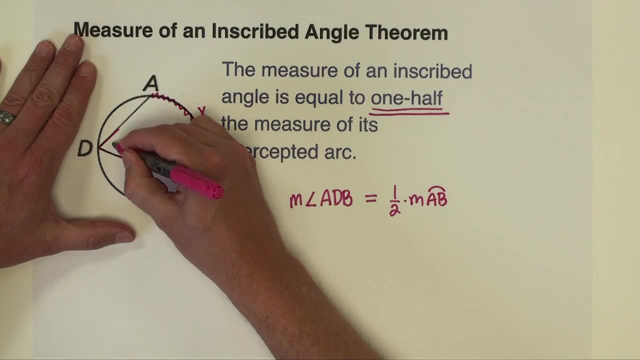 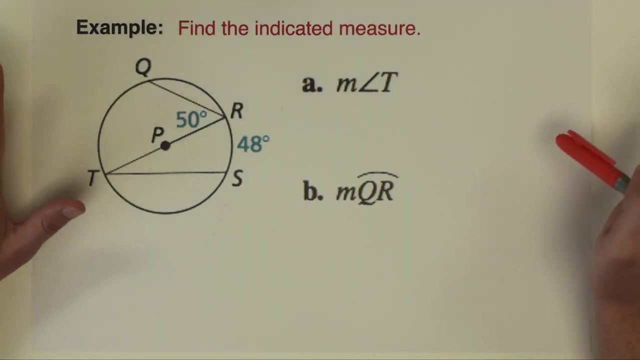 on the diagram. if I know that the measure of this arc is, say, X, then that means the measure of this angle right here is half of X. Okay, now for a couple of example problems to test out and practice that theorem. We're asked to find the measures of angle T and to find the measure of arc QR. So starting, 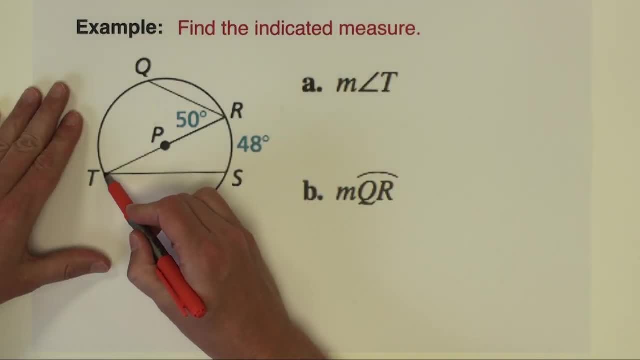 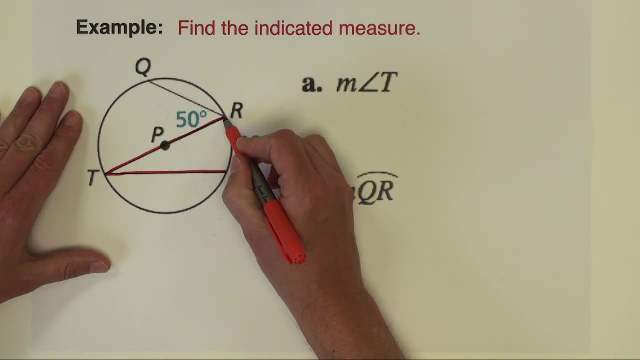 with the measure of angle T. So angle T on this diagram is right. here It is an inscribed angle. I notice that the sides of this angle intercept an arc that is 48 degrees. According to that theorem, the measure of this angle should be: 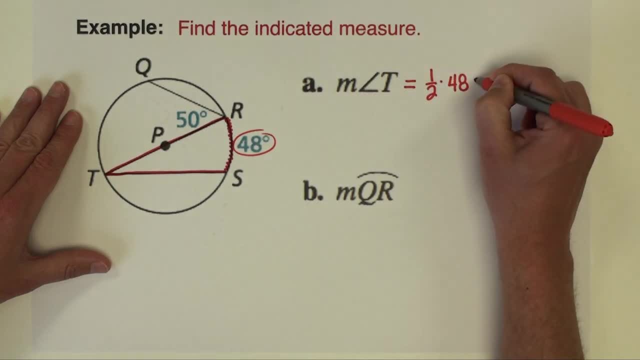 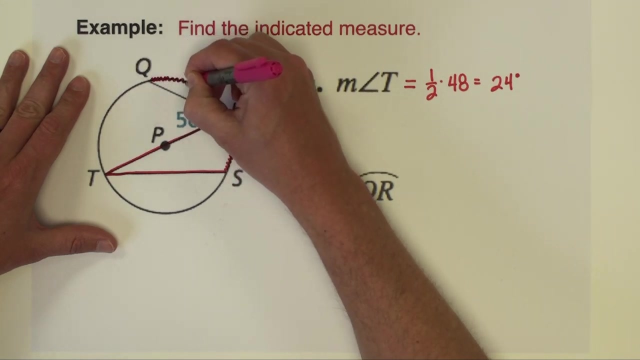 half of X, half of that arc, So it should be half of 48 degrees, which is 24 degrees. Okay, next problem: we want to find the measure of arc QR. So arc QR, that's over here. Notice that there is no. 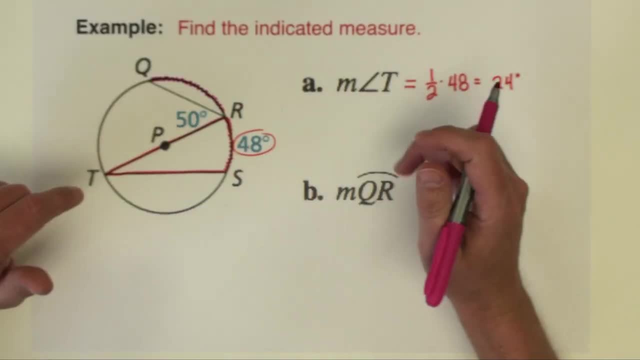 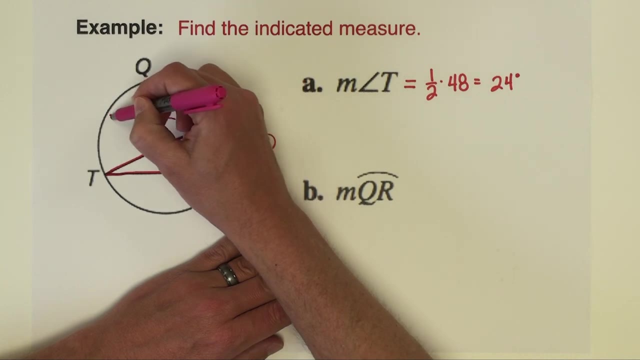 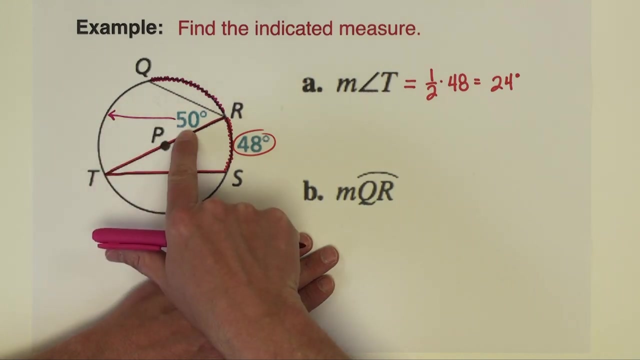 inscribed angle anywhere that is intercepting that arc. But we do have this other angle, this 50 degree angle, and this 50 degree angle intercepts that arc. Well, if the angle has to be half the arc, that means the arc has to be double the angle. So by double 50, that means arc. 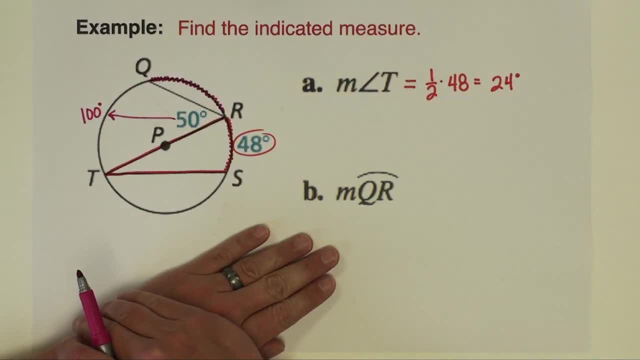 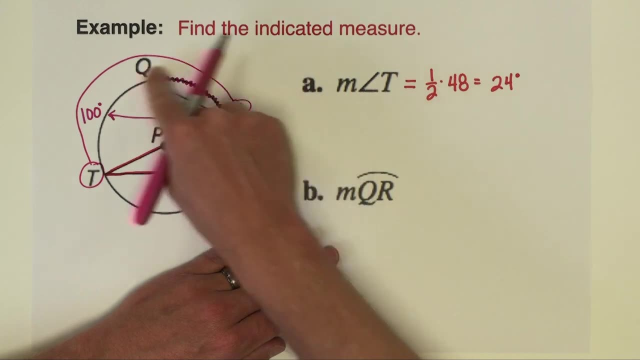 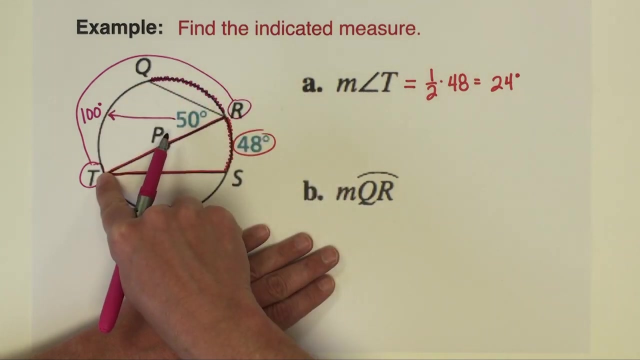 QT has to be 100. And then, looking from point R all the way around to point T, Well, that's half the circle, because RT is the diameter. So we know that the arc from R to T has to be 180.. So we can find the measure of arc QR if we do 180 minus 100. 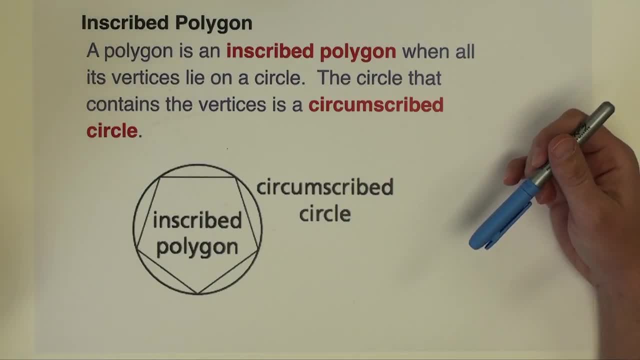 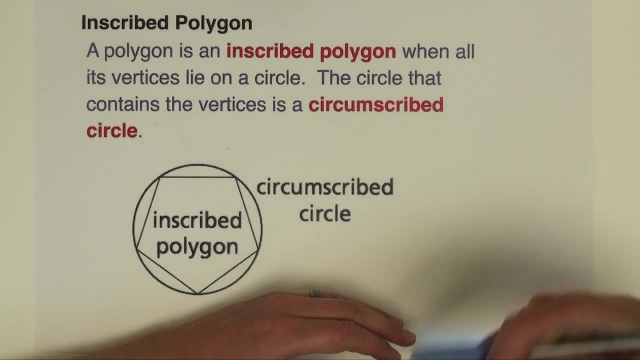 That arc is 80 degrees. Next up let's look at a little bit more vocabulary And then we'll hit you with a couple more theorems and example problems that will support those theorems. First one is just an extension of where we started in this video, And that is we're. 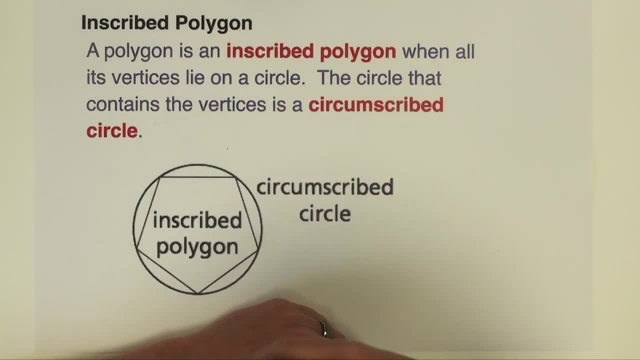 going to talk about inscribed polygons. Now, if we know, an inscribed angle is one where the vertex is on the circle. So say, this angle right here, who has its vertex on the circle? Well, an inscribed polygon simply has all of its vertices that are going to lie on the circle. So this vertices on 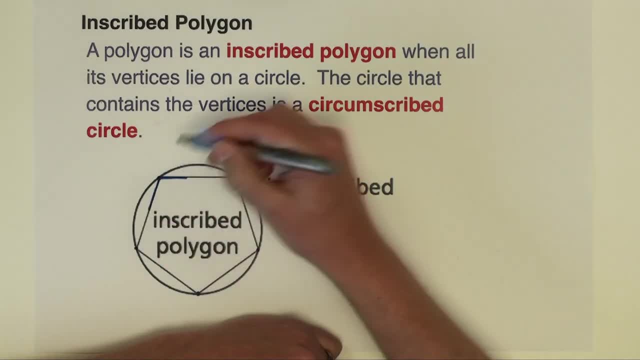 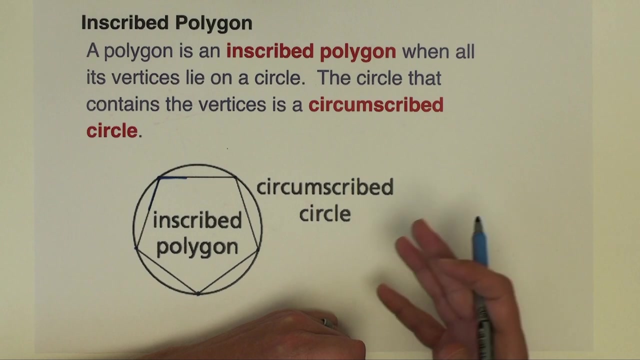 the circle: this one, this one, this one, et cetera. So every vertice is inside the circle And we call that an inscribed polygon. We can inscribe triangles, quadrilaterals, pentagons, like in this picture. Any shape that we want or any polygon that we want can be inscribed. 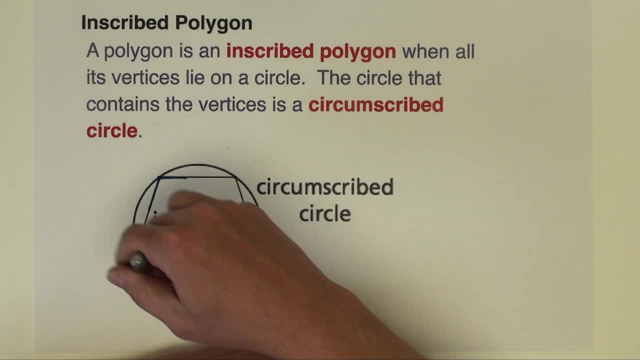 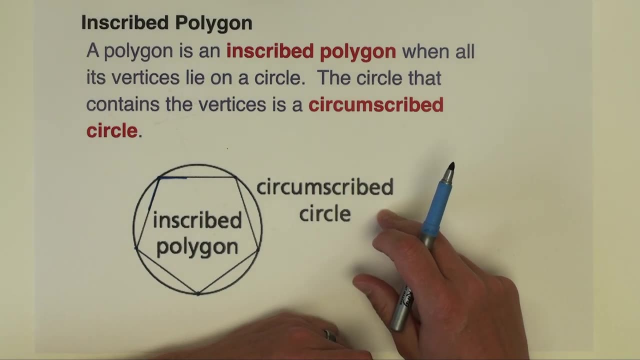 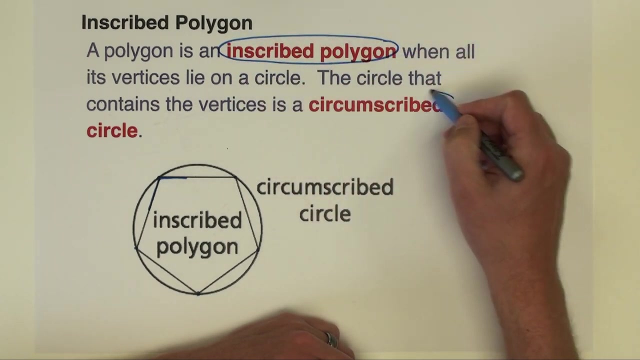 inside the circle. When we do that and the circle is on the outside of the polygon, we say that the circle that contains those vertices is a circumscribed circle. So there are a couple of definitions that we need to know: Inscribed polygon. what is circumscribed? 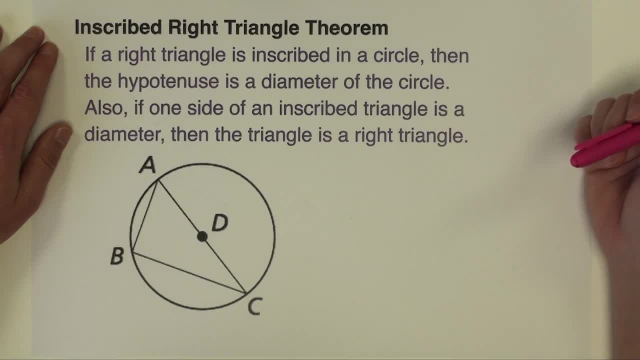 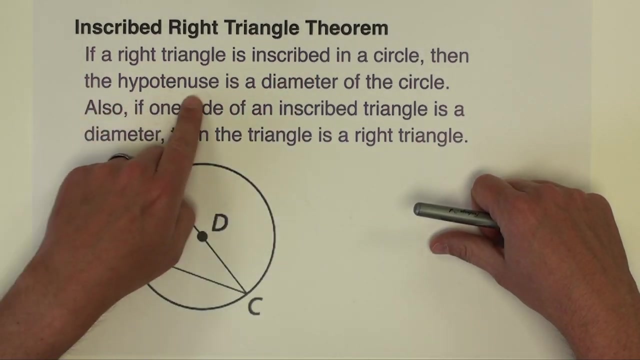 Circumscribed circle is The first theorem that we have relating or talking about inscribed polygons is called the inscribed right triangle theorem, And this theorem says that if a right triangle is inscribed in a circle then the hypotenuse is a diameter of the circle. That part. 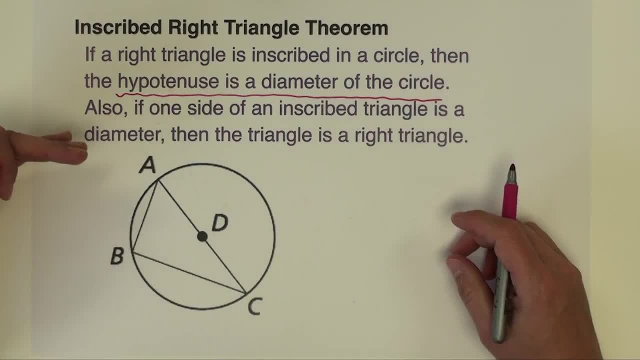 right. there is the important part Also. we can kind of reword this. conversely, It says that if one side of an inscribed triangle is inscribed in a circle, then the hypotenuse is a diameter of the triangle. So the triangle is the diameter. then the triangle is a right triangle. The reason why. 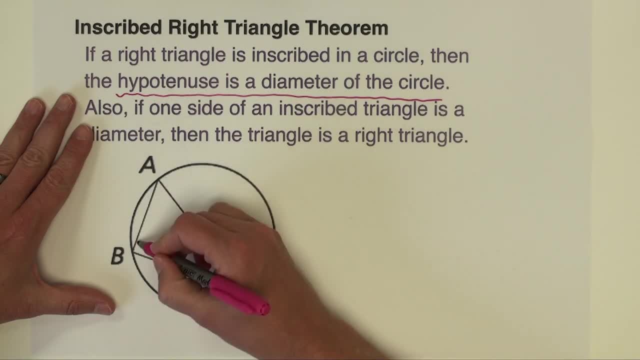 this works if we have a right triangle. so if this angle right here is 90 degrees and the sides of that angle are hitting at A and C, well, that means that the arc between A and C is 180 degrees. It has to be double what the angle is. 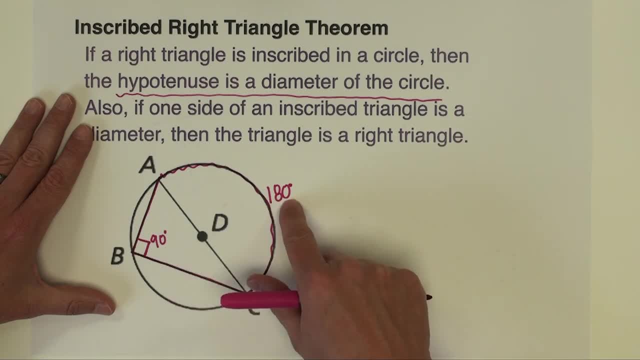 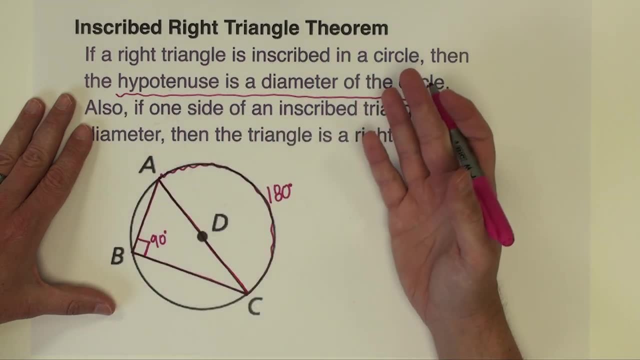 previously mentioned in this video. If this is 180 degrees, then that means that this cord from A to C is dividing the circle in half, because 180 is half of 360.. That makes AC, right here, a diameter of this circle. All right, let's look at an example problem that illustrates the theorem that we just 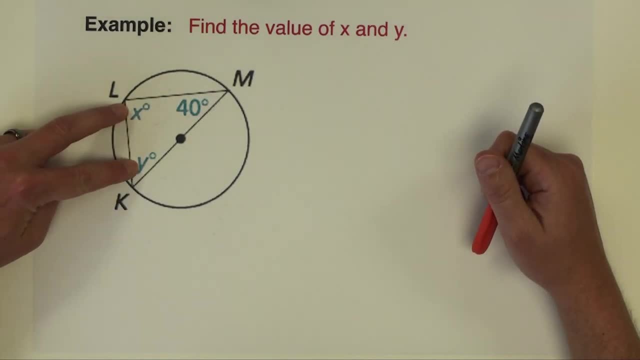 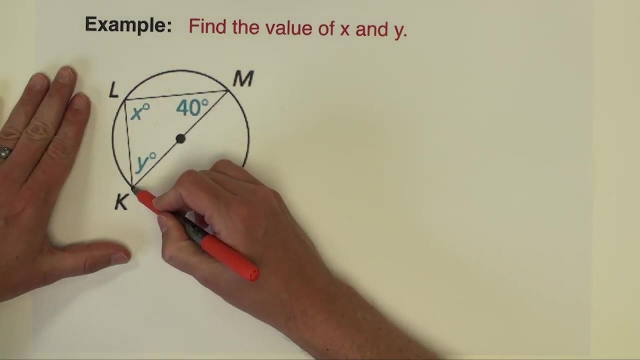 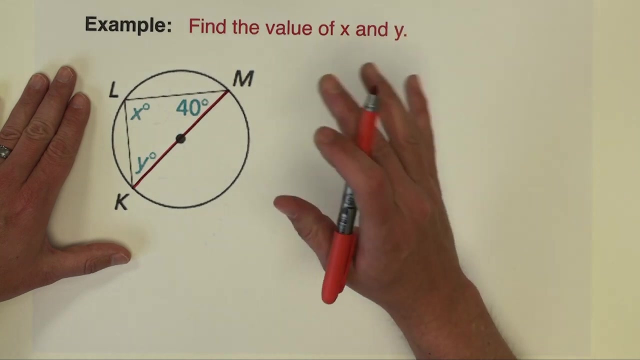 talked about Directions here are to find the value x and y in the picture. First thing that I notice in looking at this is that from K to M, this is a diameter. If it's a diameter, then according to the theorem, that means that this triangle that's inscribed inside the circle 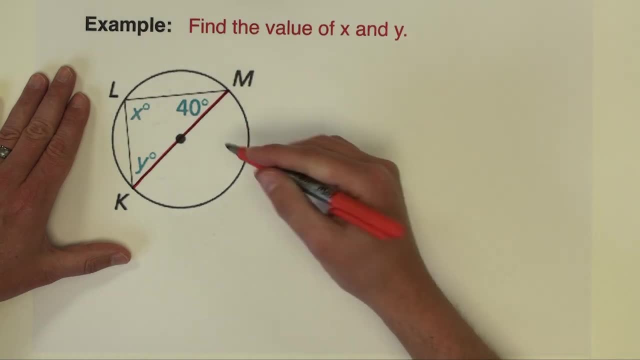 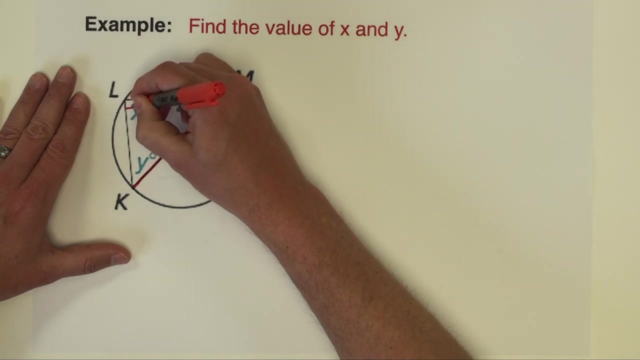 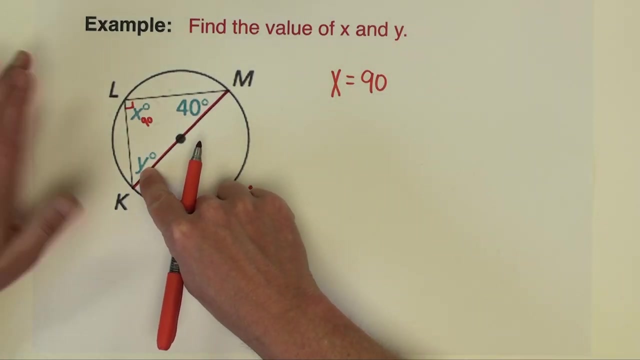 is a right triangle. Again just to support that, if it's a diameter, that means that the arc from M to K right here, is 180 degrees, which means the inscribed angle is half of that 180.. 180, which would make X 90.. Now let's look at Y. Y is now just simply the third angle in a 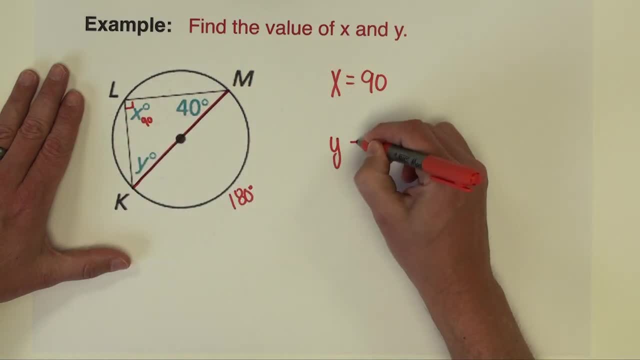 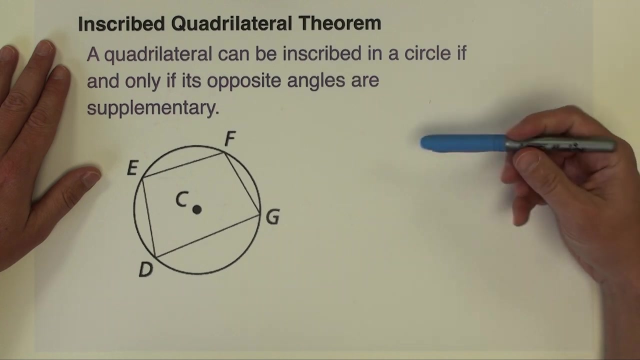 triangle where two angles are known, which means that Y can be found by doing 180 minus 90 minus 40. So Y is going to be 50 degrees to complete that triangle. The final theorem in this video is titled the inscribed quadrilateral theorem. It says that a quadrilateral can be inscribed in a. 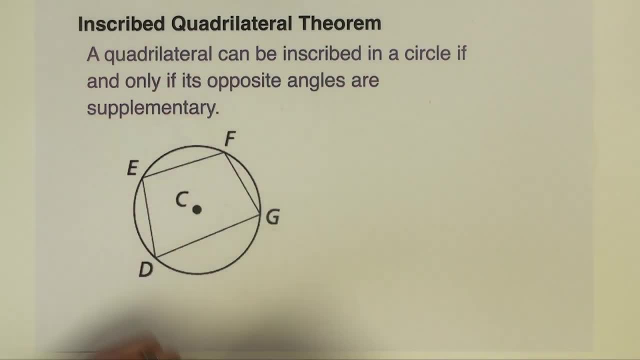 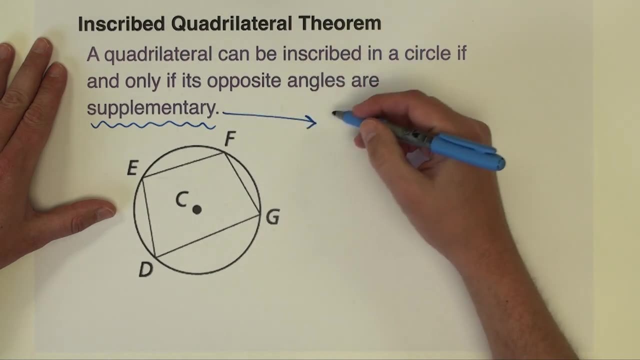 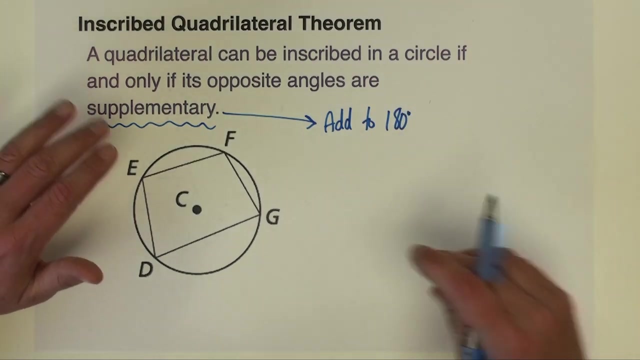 circle if, and only if, its opposite angles are supplementary. So we know what that means. Supplementary means that those angles add to 180 degrees. Well, let's take a look at that. If I were to look at. we need some opposite angles. So let's look. 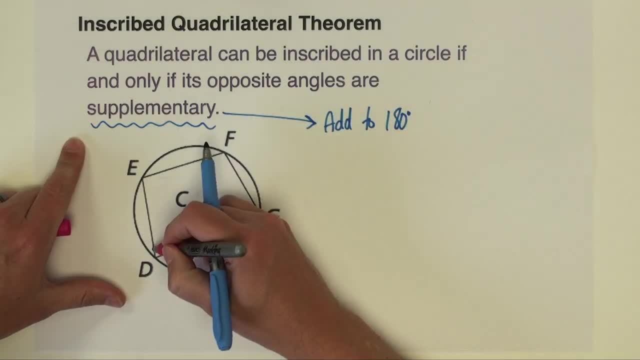 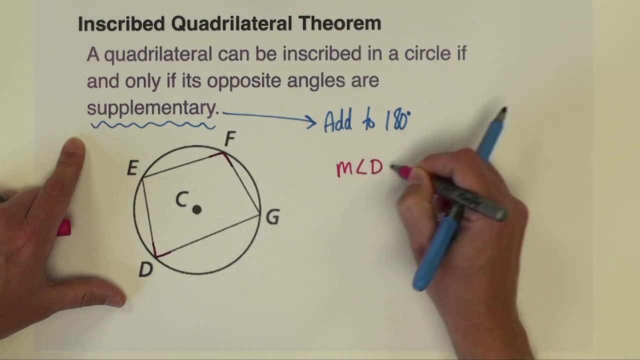 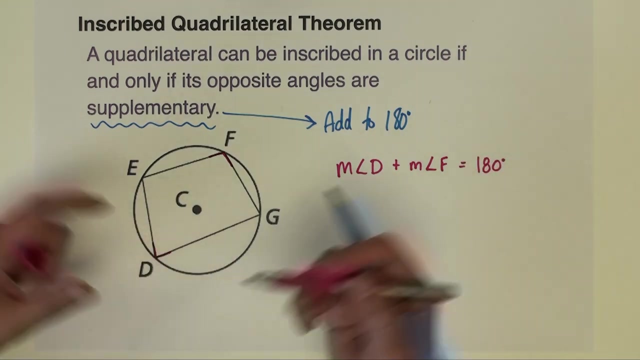 at angle D and angle F. According to this theorem, angle D right here- and angle F are going to add to 180.. Let's see why that works. If I extend the sides of angle D until it hits the circle, it intercepts this arc right there, If I 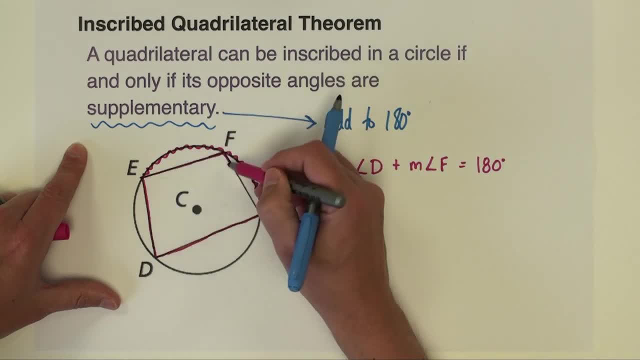 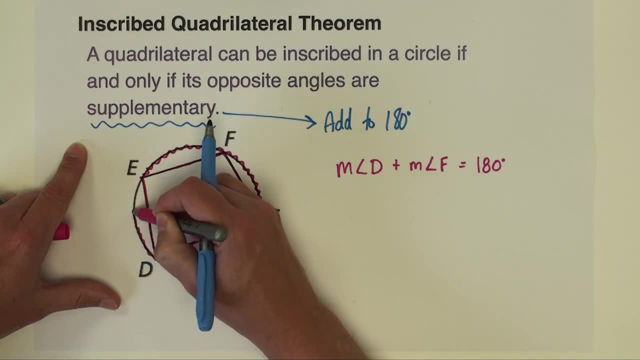 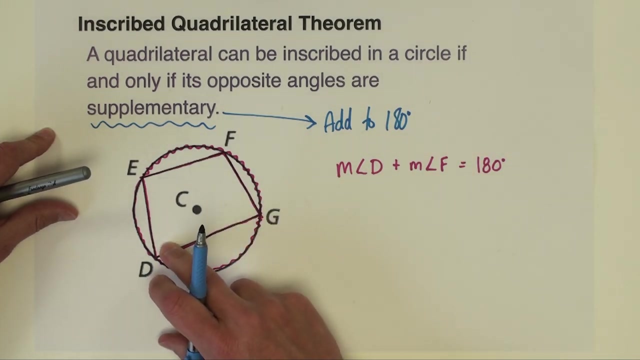 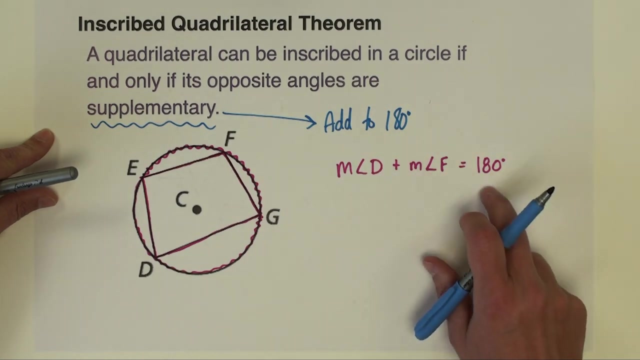 extend the sides of angle F to where it hits the circle. I have intercepted that arc. notice that the intercepted arcs are now the entire circle. we know that the entire circle is 360 degrees and that the inscribed angle, or in this case angles, have to be half of the intercepted arc. so half of our 360 is. 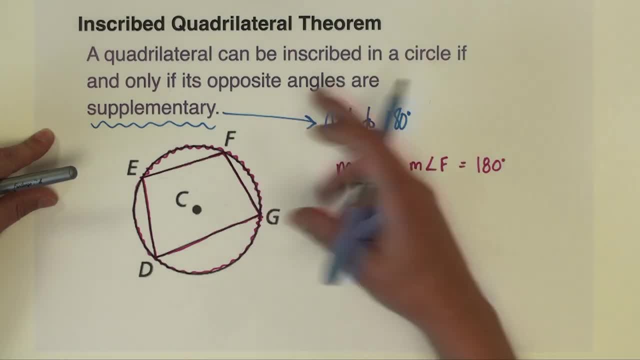 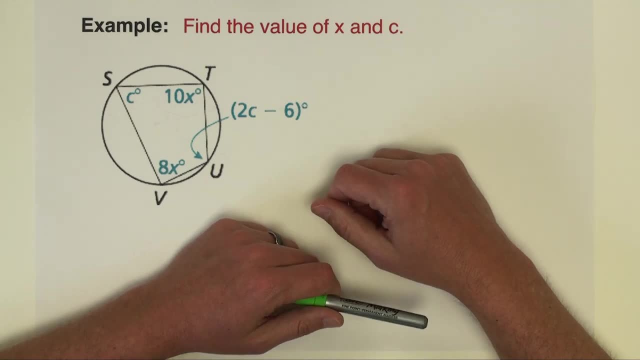 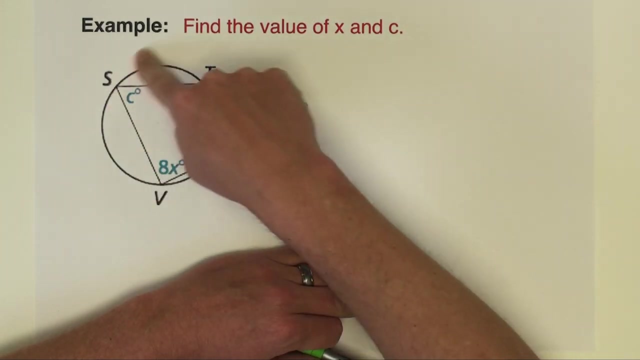 the 180. that's why this theorem works all right. let's look at one example problem to illustrate this theorem. directions in this example problem are asking us to find the value of X and C. when I look at this, I notice that I do have a quadrilateral that's inscribed inside the circle, which means that